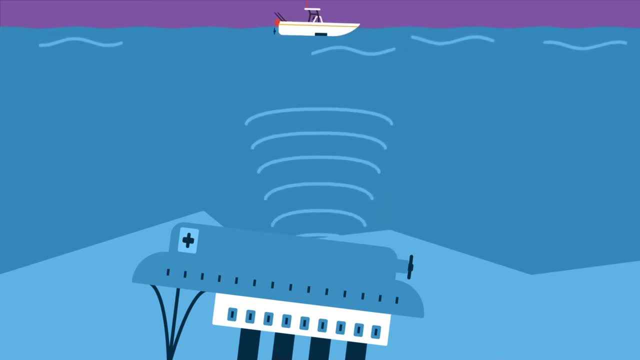 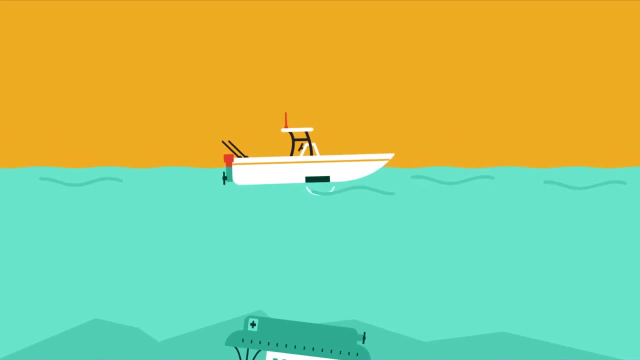 off a submerged object to find and determine the depth of an object which is invisible from the surface. The surface ship is often called the Titanic. The Titanic is called the Titanic because it is the ship of stars that are in the sky, sends out a sonar pulse, a sound wave, into the water. It travels away from the ship until it. 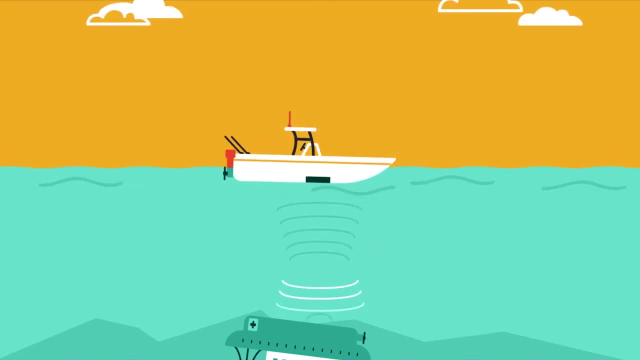 is reflected by an object in the water, The sound wave reflection, or echo, travels back up through the water and is detected by the ship. As we know the speed of sound in water, which is about 1500 meters per second, then the time lapse between signal transmission. 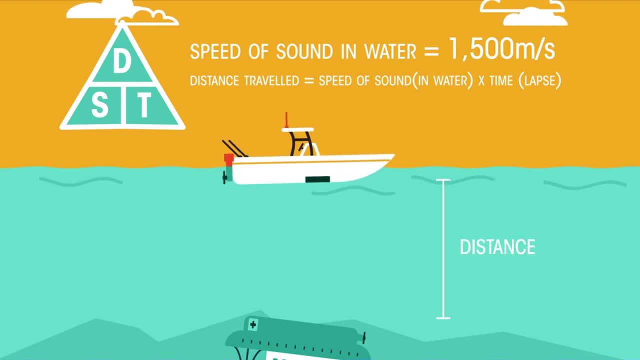 and echo reception can be used to calculate the distance the sonar wave traveled. We then divide this answer by two. You are probably wondering why That's because the first answer gives us the distance between the sender and the shipwreck and then back to the boat. We only wish to know half this distance between the sender and the 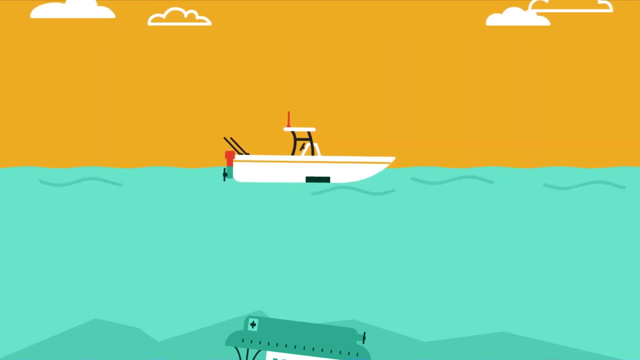 boat. If a ship above the Titanic uses sonar to detect the wreck and records a time lapse of 400 meters per second, then the distance between the shipwreck and the shipwreck is 5 seconds. How deep is it? Pause the video while you work it out. 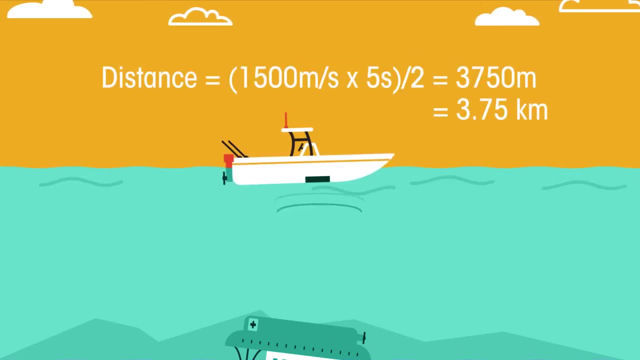 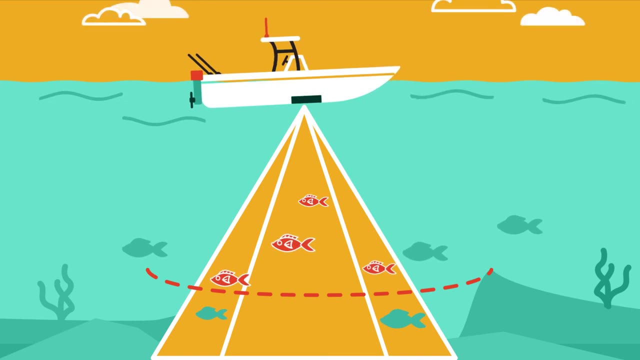 Did you get 3750 meters or 3.75 kilometers? Sonar can be quite sophisticated. Fishing boats use it not only to find fish, but can also tell the type or size of fish. To summarize, you have seen how we can use sound waves in water. 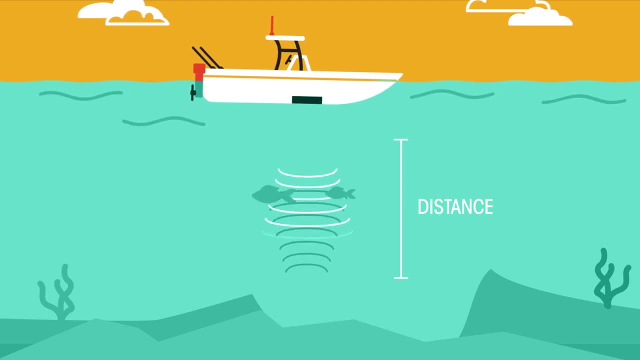 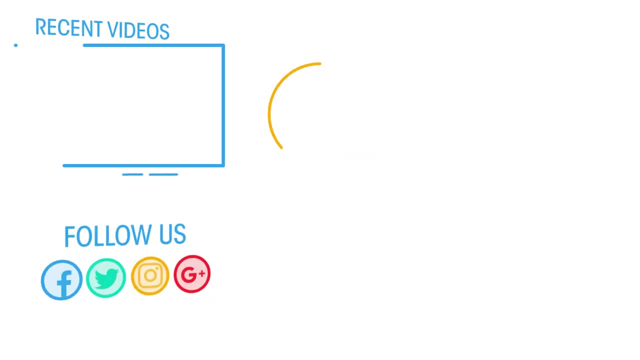 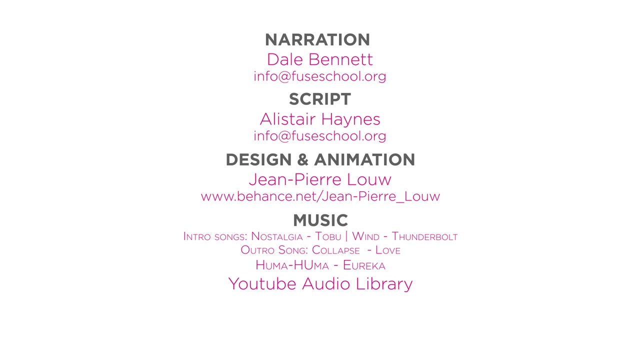 to find out where the ship is and their echo to work out the distance. something is beneath the surface. This sonar can find shipwrecks or shoals of fish. So is this the best answer? If you enjoyed this video, please subscribe, like and leave a comment. Also, if you want to see more of our videos, please check out our website. Thanks for watching and see you next time.